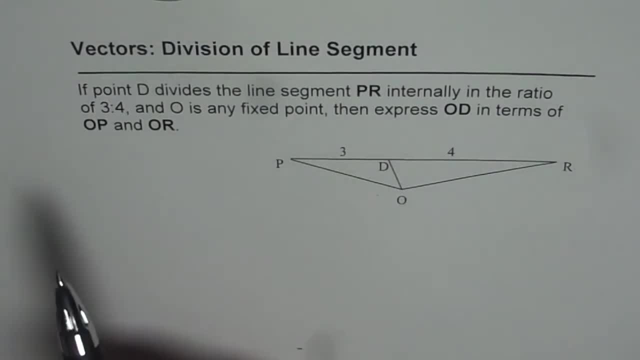 in terms of OP and OR. So what we are given here are two points, P and Q. They are divided by a point D in the ratio of 3 to 4.. Now, from an external point, O, we need to express OD in terms of OP and OR. Well, in some cases what we can do is we can consider O as the 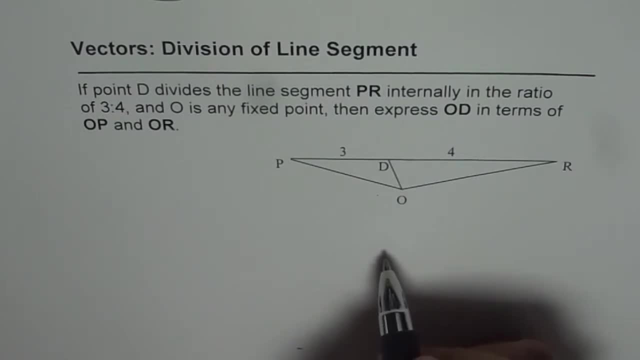 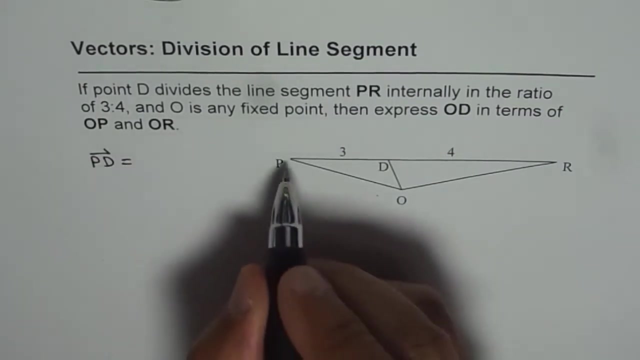 origin, then OD will be the position vector. Therefore, point D can be found in this fashion. So that is an application which we are going to do in the following videos. Now let's try to relate OD with OP and OR. Now from this figure we can say PD vector. PD is a ratio of total length which is 7. 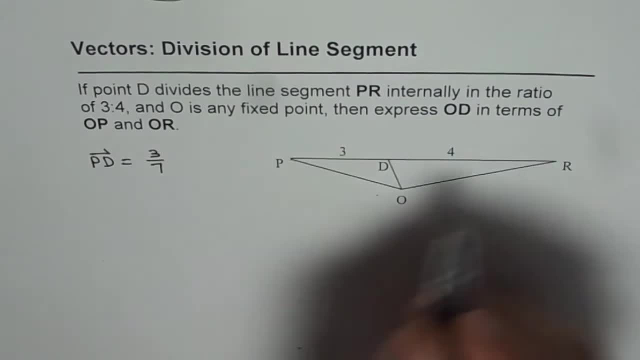 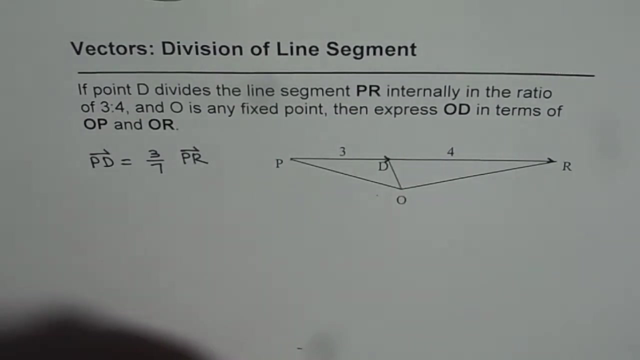 to 3.. It is 3 over 7.. So this is the total length of PR, correct? So PR, that is PD and this is PR. Total length is 7 and PD is only 3 parts of the total 7.. So that is known to us. 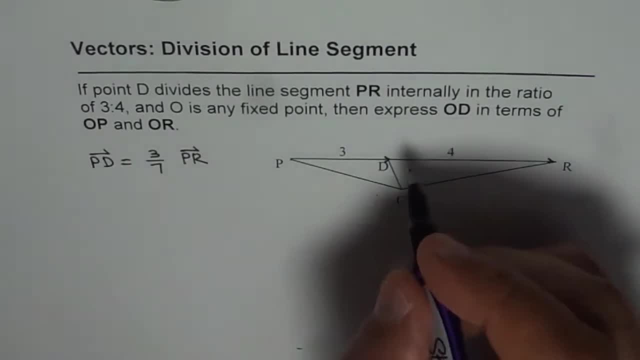 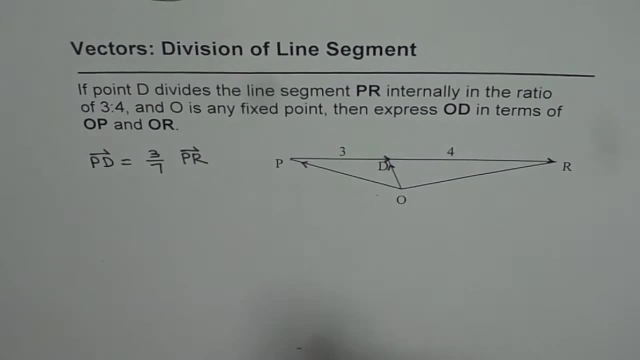 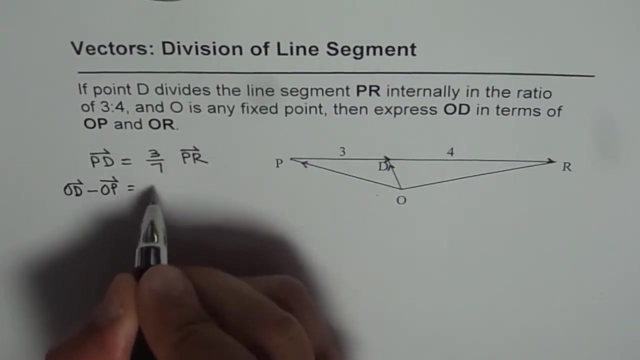 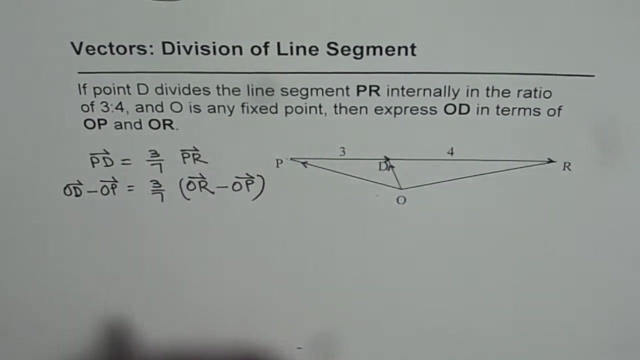 Now, what is PD? PD can be written as OD minus OP, correct? So we will write PD as OD minus OP. 3 over 7 and similarly, PR P to R can be written as OR minus OP. That is OR minus OP We need. 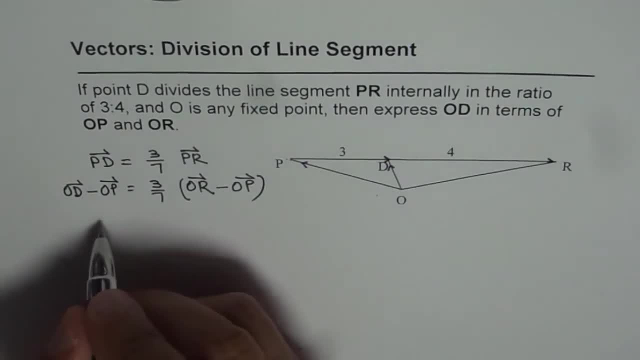 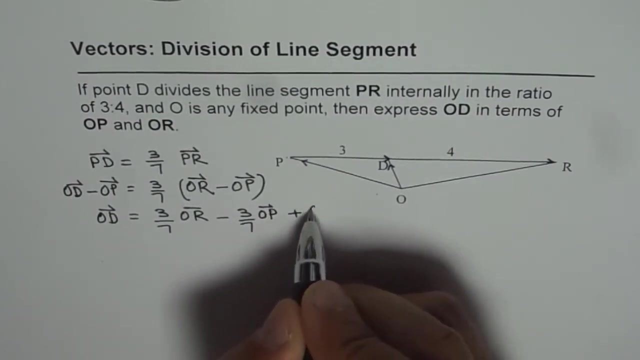 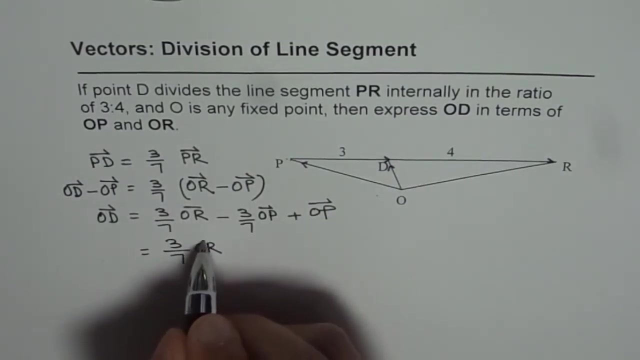 to find what OD is. So let's take OP on the right side and find what OD is. So OD is equals to- let's open this bracket also- 3 over 7 of OR minus OP, 3 over 7 of OR minus 3 over 7 of OP. That gives us 3 over 7 of OR, and let's add these: 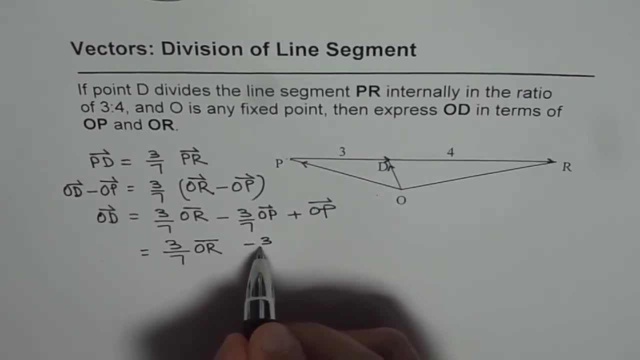 together, so we get minus 3 over 7 OP. We can write this as plus 7 over 7 OP, Just common denominator right P plus 7 over 7 OP. now that gives us 3 over 7 of OR and this is 4 over 7 of OP. so that is how OD is related. 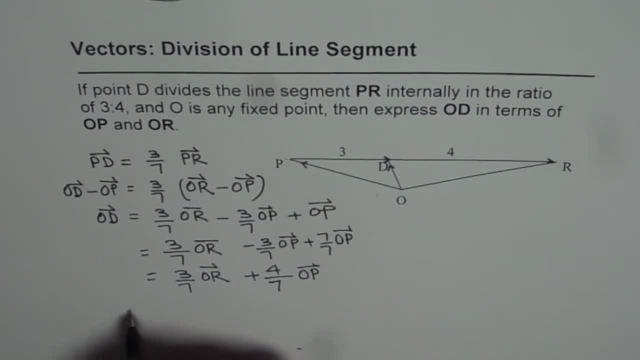 right with OR and OP. so now I can write this as kind of a formula: for us, OD is equals to 3 over 7 of OR plus 4 over 7 of OP, correct? so that is how they are related. now let me generalize this formula here. we will do separately. also, let us say that the ratio in which it 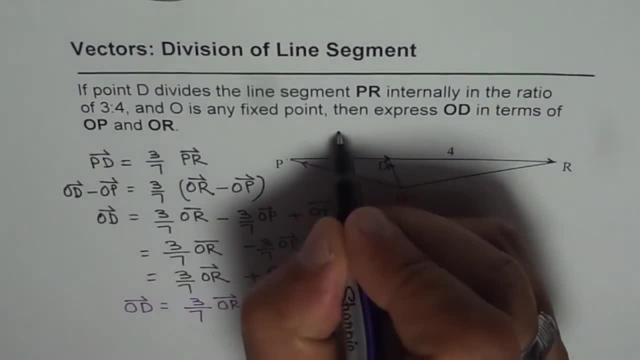 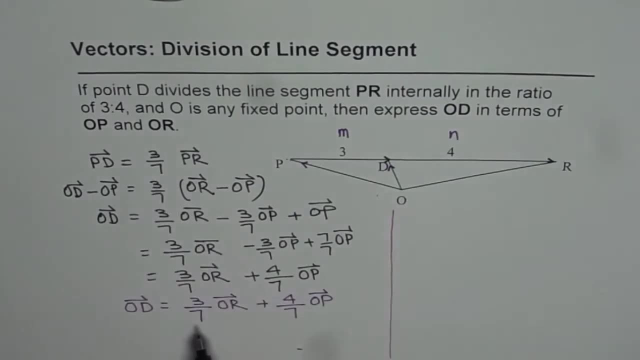 divides is actually M is to N instead of 3 and 4, if we take M and N. in that case, if you redo all these calculations, replacing 3 with M and M, plus N as 7, right and 4 as N, right, so what do you get? you get a formula which is: OD is equals to 3 as M divided by 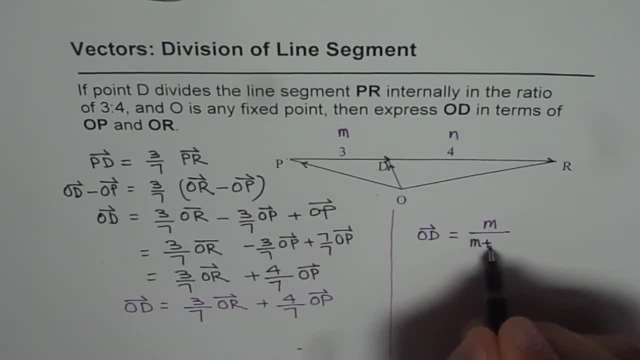 7 is M plus N OR plus 4 over 7 of OP, right? so that is how they are related. now let us say that 4 is N, right, M plus N over P. so that is a general formula which you can apply for internal division, right? let me also make a note here for external division, what we should. 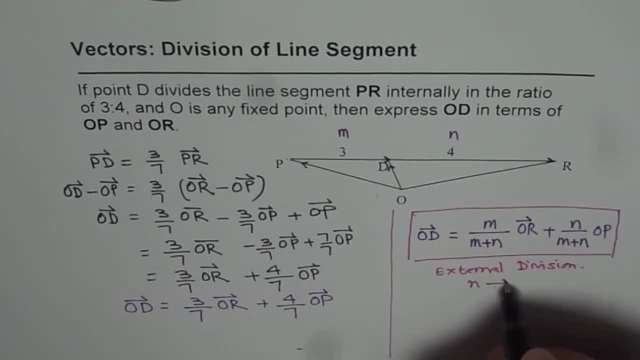 do is we can replace N with minus 4.. So that is a general formula which you can apply for internal division, right? let me also make a note here for external division: replace N with minus N, right? what we'll talk about external division later. it really means that if this is my P and R, then the point D is outside, right, and in that case when we say M to N, we say this is M for us and this ratio is N now, since it is in the reverse direction we are taking. 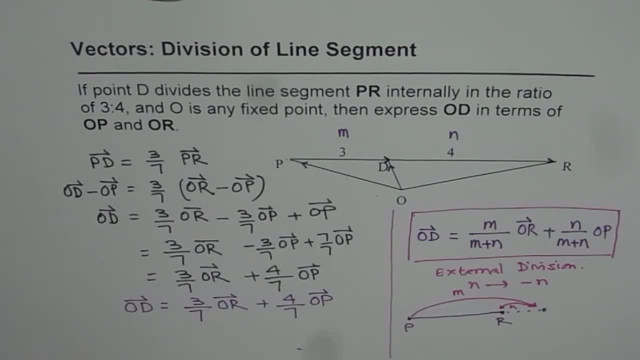 it as minus n, the same formula will work right. So what I will advise you to do at this stage is derive these two formulas correct. So derive these two formulas. that will give you good confidence and some practice on similar questions. Thank you and all the best.